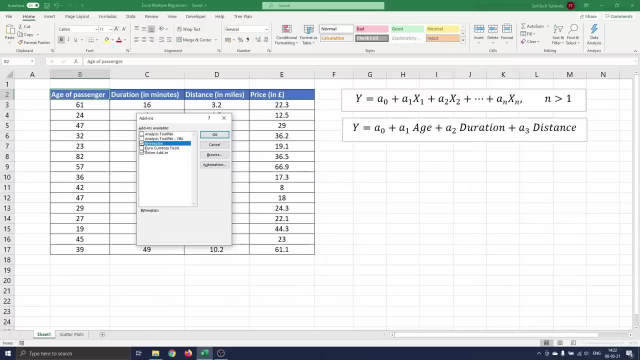 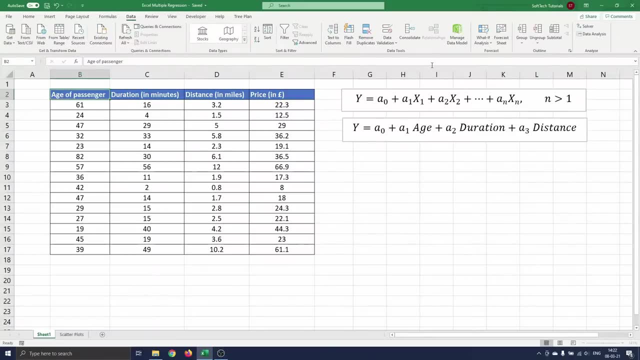 Here. you make sure the checkbox next to analysis tool pack is checked and you press on ok. Now you can see under data that data analysis is added. You click on data analysis and select regression. A menu opens where you can insert the dependent and all independent. 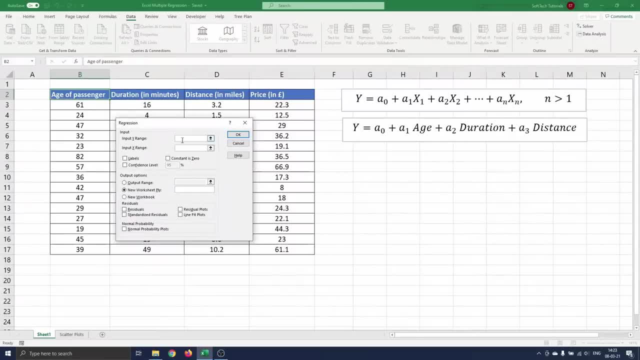 variables. The y-range represents the dependent variable, so we select range E2 to E17.. The x-range represents the independent variables which are loaded in columns B, C and D, So we select the range B2 till D17 as inputs for the x-range. 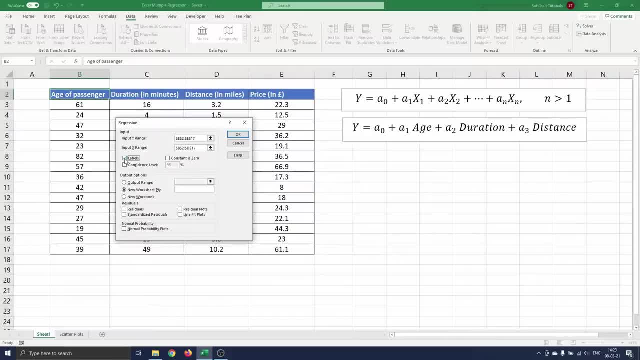 We have also included the labels in the ranges, so we tick off the labels box Before we click on ok. we choose a location in the workbook where we want the analysis to appear. We want to make it appear next to our input table, so we select G2.. Click on ok and you see the analysis. 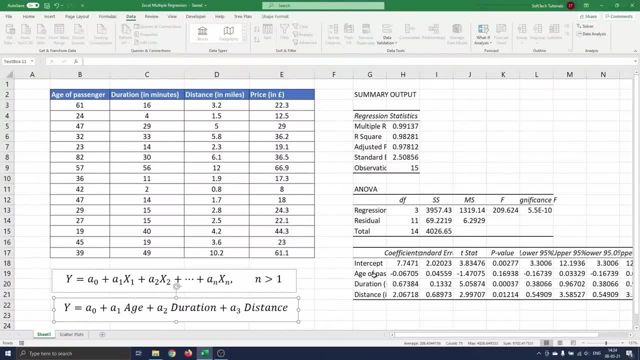 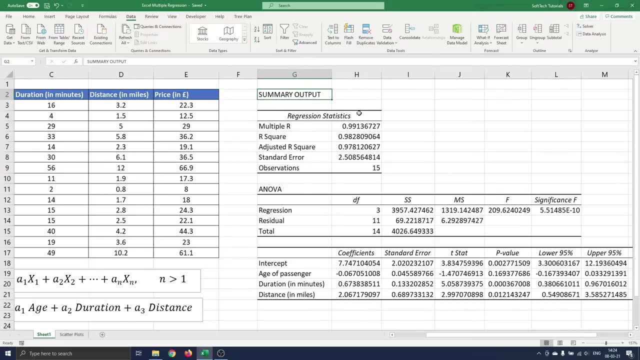 output appear on the screen. We want to make it appear next to our input table, so we select G2.. Click on ok and you see the analysis output appear on the screen. The output of the analysis is divided into three parts. First we have the regression statistics that tell you how well the calculated linear regression 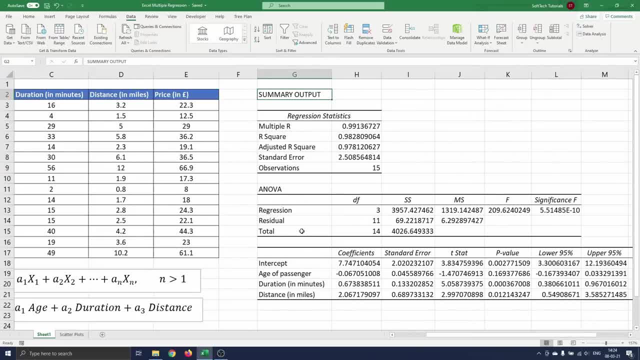 equation fits your data. The second part shows you the different components of the sum of squares and gives you an idea of how reliable the model is. The final part of the regression output represents the different variables in the regression and the linear regression equation. The most important block of output is the third one. So in this, 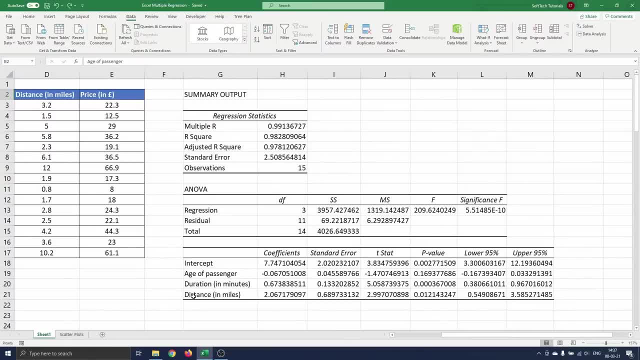 video. we will mainly focus on this, but in the other two parts I'll highlight the most important figures to see what they represent. In the regression statistics part, the most important figure is the adjusted R-square. It represents the R-square adjusted for the number of independent. 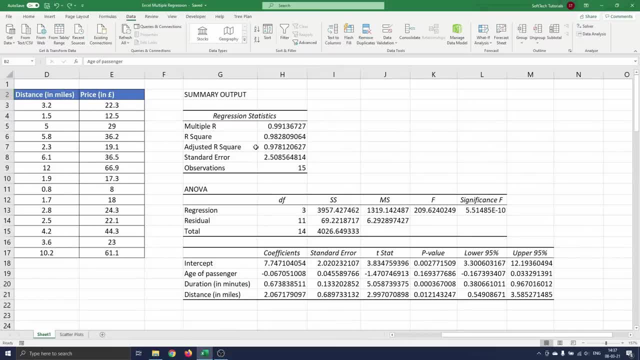 variables in the model. In the case of multiple regression, you always want to use this form of the R-square. In our example, this figure is 0.978, which means 97.8% of the number of independent variables. In the case of the R-square, the R-square is 0.098% of the observation of the dependent variable. are: 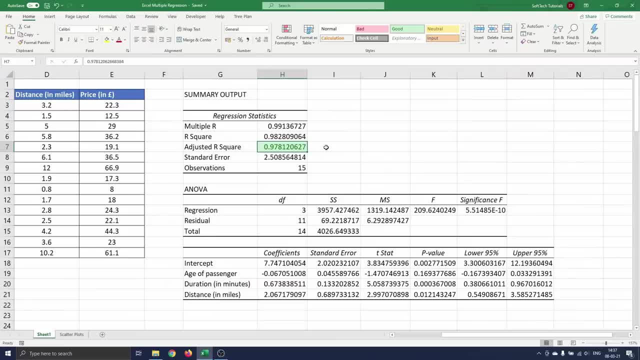 explained by the independent variables. This figure is higher than 95% and hence considered a good fit. The ANOVA table shows the reliability of our model. The most important figure in this context is the significance f-value, which is the probability that all regression coefficients. 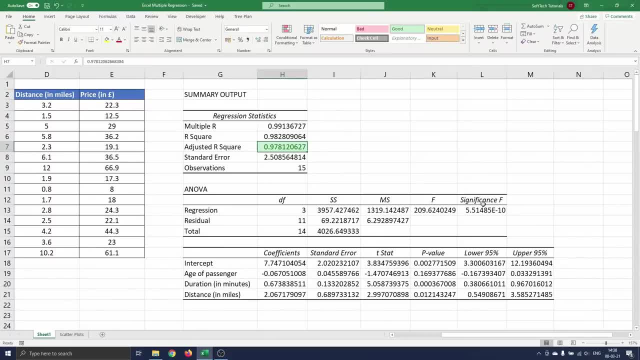 are 0.. In other words, we test the reliability of the entire model. When the significance f is, We reject the null hypothesis that all regression coefficients are zero and we can say that the model is reliable. In our case, the significance F-value is well below that threshold, so we can. 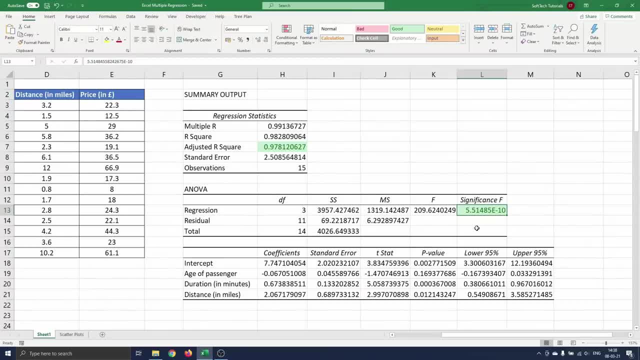 conclude that our entire model is relevant for our data. The first column in the third table gives the estimated coefficients for the regression equation. The second column, standard error, gives the standard errors or estimated standard deviations of the least squares estimates. For the third column, we first have to say that Excel performs hypothesis testing. 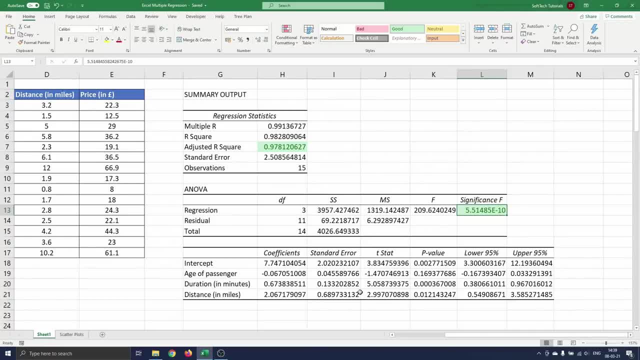 for each regression coefficient. Excel tests the null hypothesis that the coefficient is zero. The t-stat and p-value columns show the corresponding t-statistics and p-value for these tests. The last two columns show the 95% confidence interval for the regression coefficients. 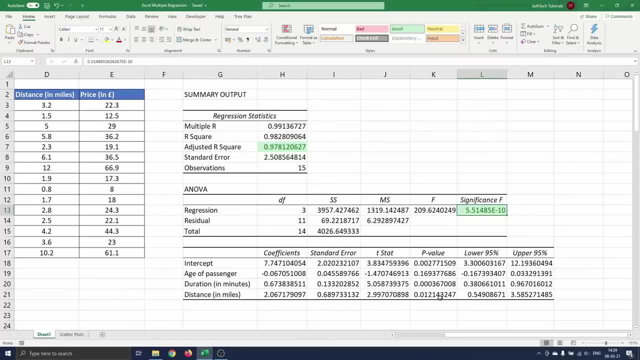 Now we focus on the p-values, as these are the most important figures, besides the regression coefficients. Now we focus on the p-values, as these are the most important figures besides the regression coefficients. Now we focus on the p-values, as these are the most important figures, besides the regression coefficients. 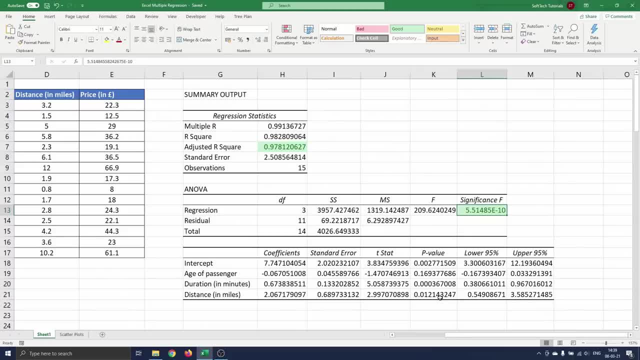 A commonly chosen threshold to say that the coefficient is significantly different from zero and hence that the independent variable is relevant, is 0.05.. We say that all values are lower than 0.05, except for the one of the age. This is something we could expect as the age of. 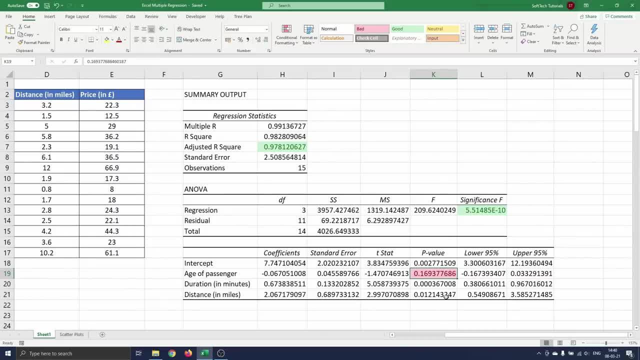 a person is only random and will not be an influential factor for the price of a taxi ride. Another clue for this could have been when you first created the scatterplot with a trendline for each variable. We have done this on the second excel sheet. The trendlines fit the 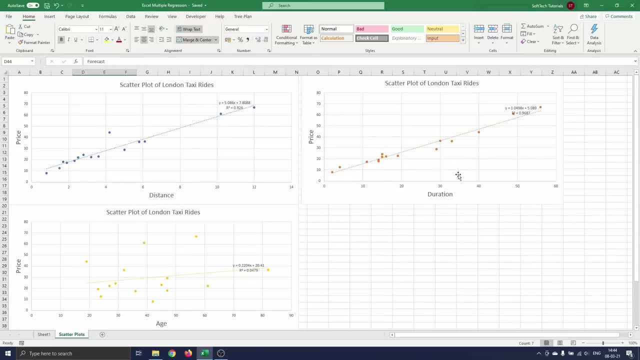 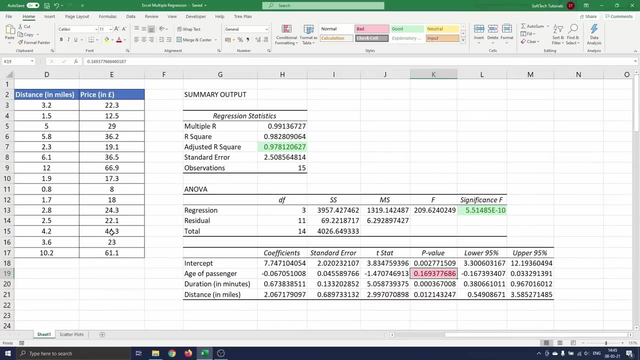 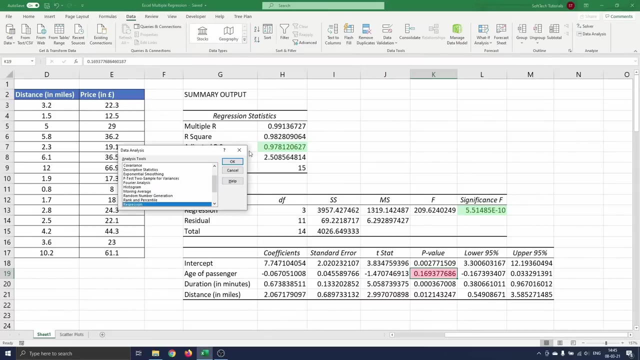 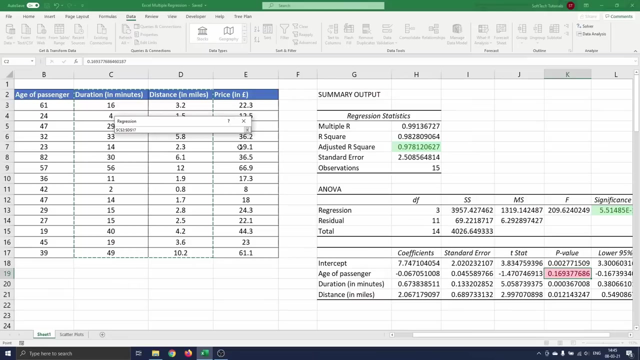 distance and duration variables nicely, in contrast to the age variable, where you see a fairly random distribution of the observations. Now that we have concluded that the age variable is not relevant, we will do the regression again without the age variable. To do so, we go back to data data analysis and change the input x-range to C2 till T17.. We put this output. 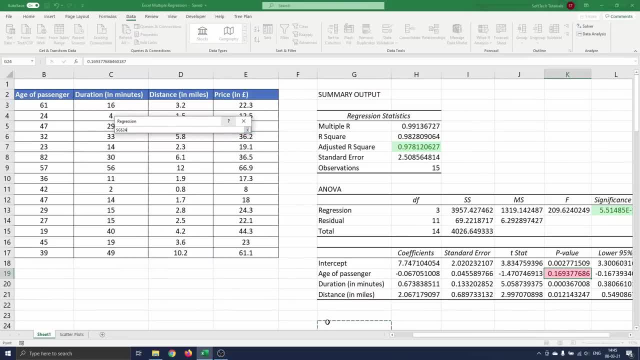 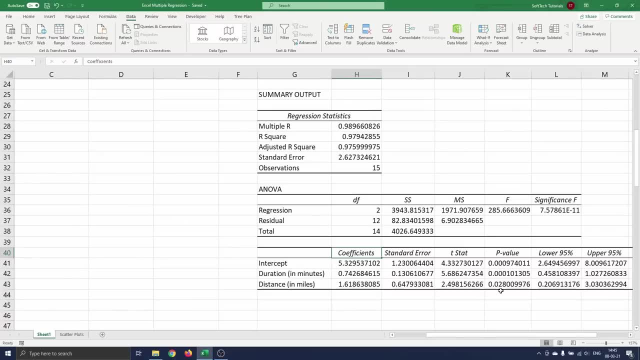 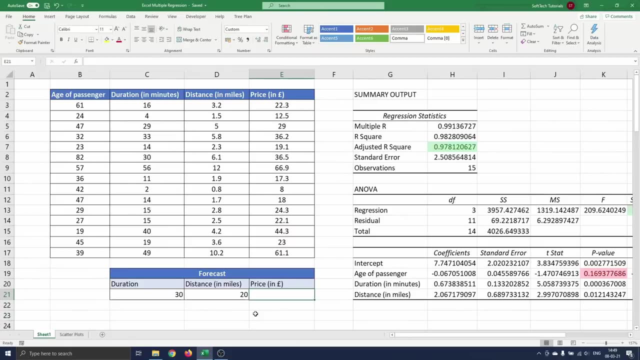 below our first output, so we select G25 as output range, We press on ok and see the output appear on the screen. The three p-values are below the 0.05 threshold now, and hence this model fits the data. well, We have defined our model and can use it to forecast the cost of our upcoming taxi ride. 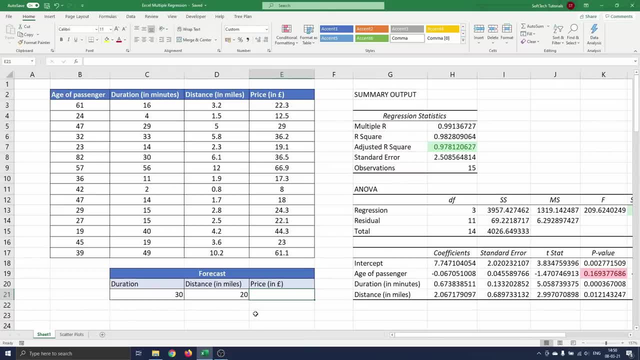 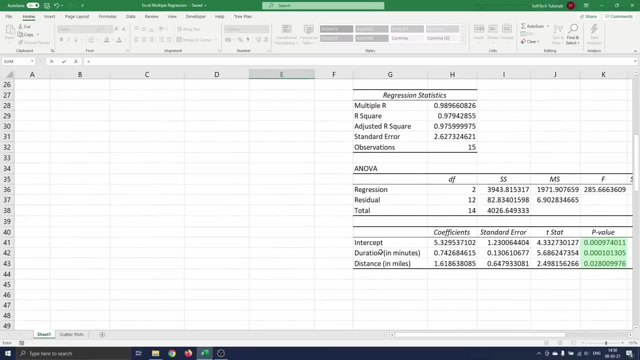 in London We need to take a cab from the airport to our hotel. This is a 20 miles drive. Our flight is at night so there won't be any traffic. We expect that the ride will continue. To compute this we type equals the coefficient corresponding to the duration variable. 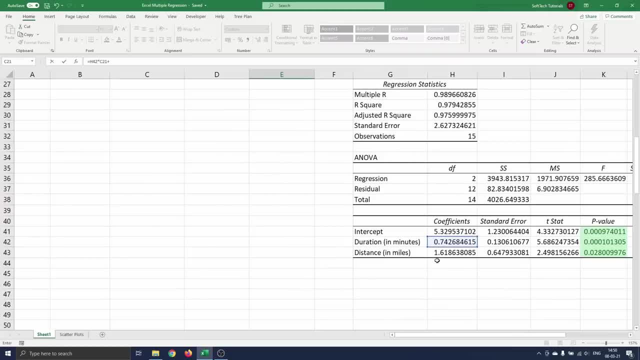 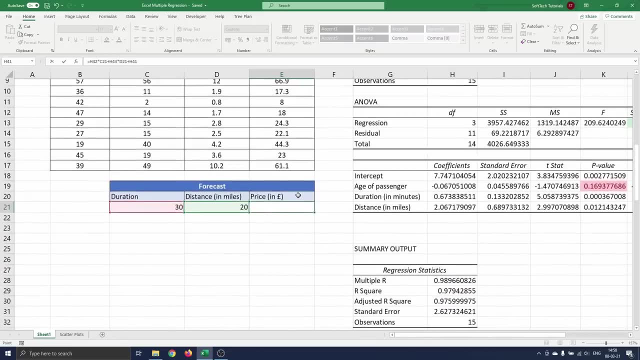 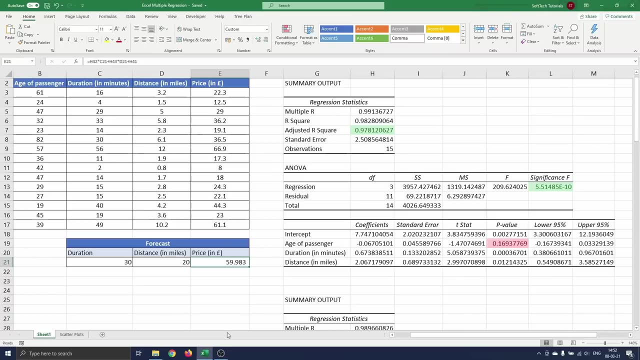 times 30, plus the coefficient corresponding to the distance variable times 20, plus the intercept, We press enter and see that the estimated cost is 59.98 pounds. This concludes our tutorial on multiple regression in excel. If you have any questions or comments, 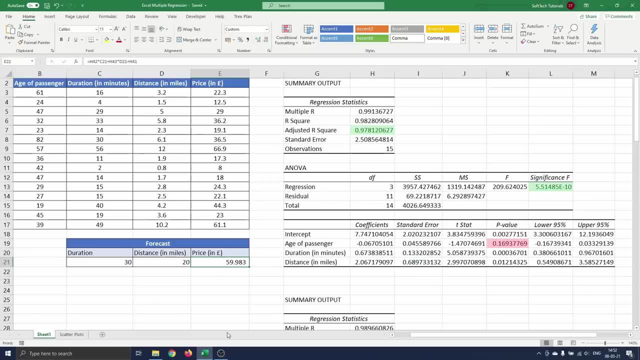 let me know. Be sure to subscribe if you want to watch more excel or software related tutorials. Thank you for watching and I'll see you in the next one. 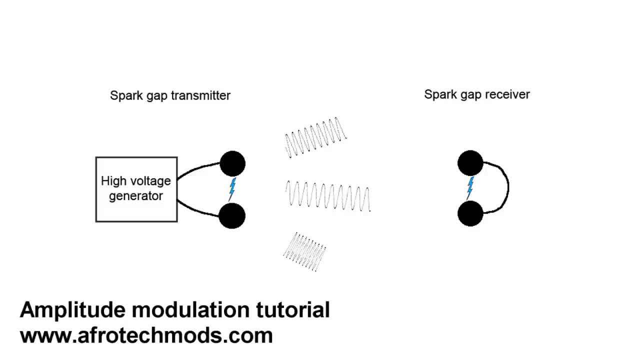 In this video I'm going to cover AM all the way from the discovery of radio waves to building your own AM radio transmitter. Heinrich Hertz was the first scientist to successfully generate and receive electromagnetic waves. He did it by creating voltages high enough to create some sparks and the 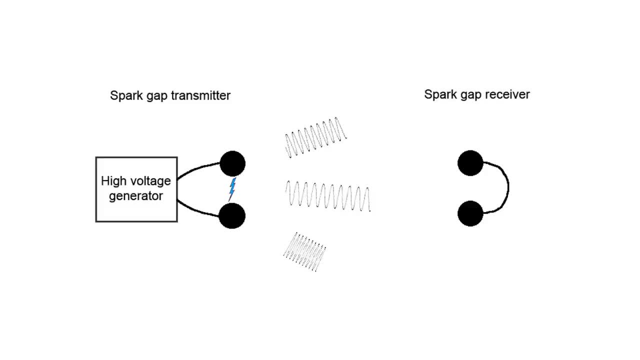 sparks emitted electromagnetic waves of all kinds of frequencies. When these bursts of electromagnetic radiation reached a receiving spark gap, another spark appeared. This experiment was pretty crude, but it was the first time anyone had communicated information via radio waves. You can replicate the experiment right at home with an AM radio and a light switch. 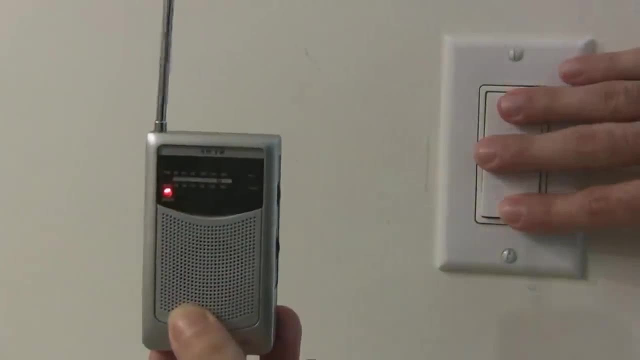 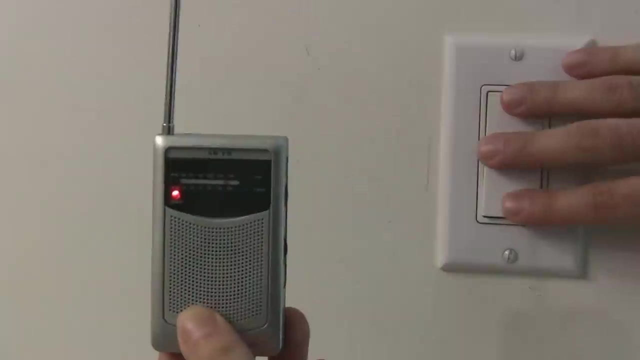 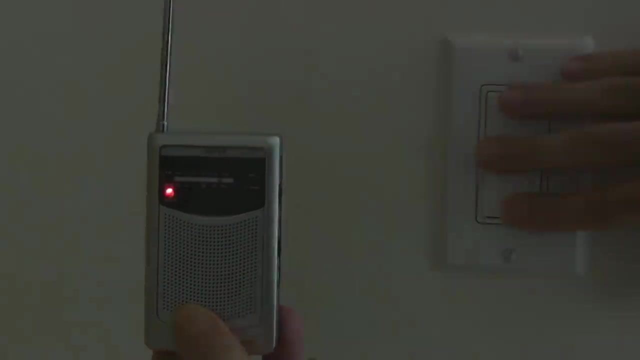 Just tune the radio to a quiet station and flip the light switch on and off. The little sparks generated when you flip the mechanical switch create a little burst of electromagnetic radiation and your AM radio detects it as a little popping noise. A few years later, Nikola Tesla created radio transmittance. 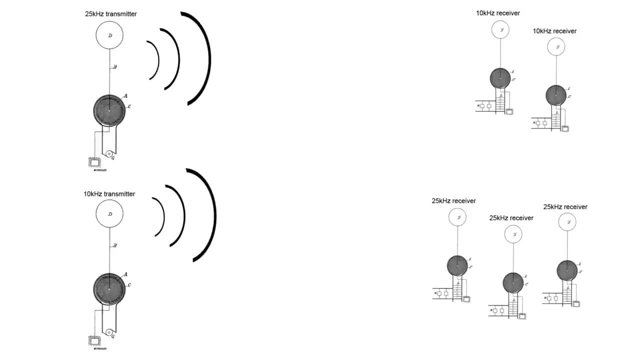 that could be tuned to different frequencies, so many people could transmit and receive information at the same time without interference. He accomplished this by creating a transmitter that was essentially a high-voltage oscillator with an adjustable frequency, and his receiver was basically a well-tuned LC filter, which. 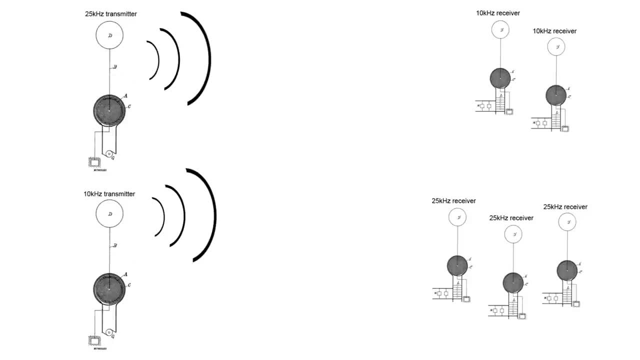 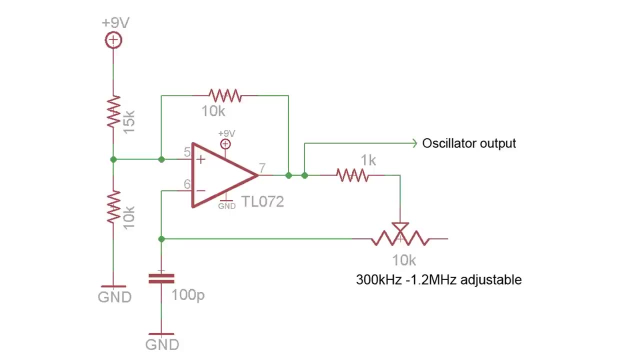 rejected all unwanted radio waves and allowed you to listen to the radio transmission you wanted. This system led to the development of telegraph machines that were used all around the world, And again you can do similar experiments at home very easily. Instead of making Tesla coils or LC-based oscillators, here's a schematic for an. 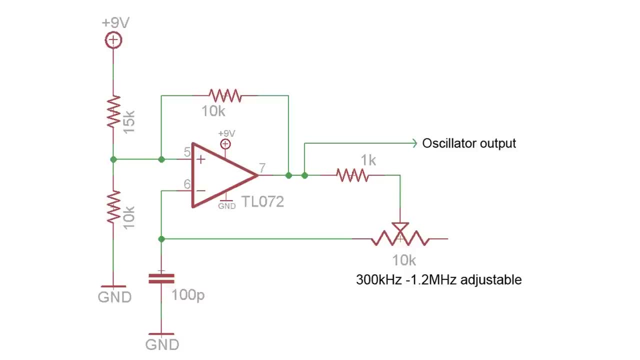 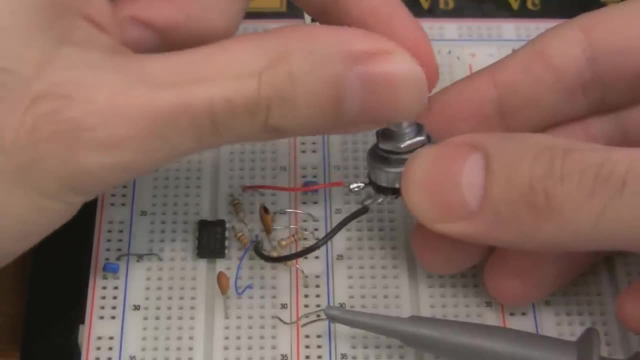 oscillator built out of an op-amp chip. It'll spit out a wave from 300 kilohertz to 1.2 megahertz and this covers most of the AM radio spectrum. If I adjust the potentiometer, I can change the output frequency I transmit on. 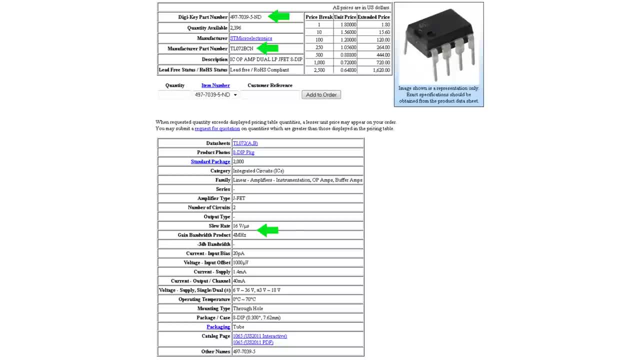 By the way, this circuit won't work with low-speed op-amps like the LM741 or LM324.. The op-amp I used is a TL072BCN that I got from Digi-Key. I'm not sure if this circuit will work with low-speed op-amps like the LM741 or LM324..